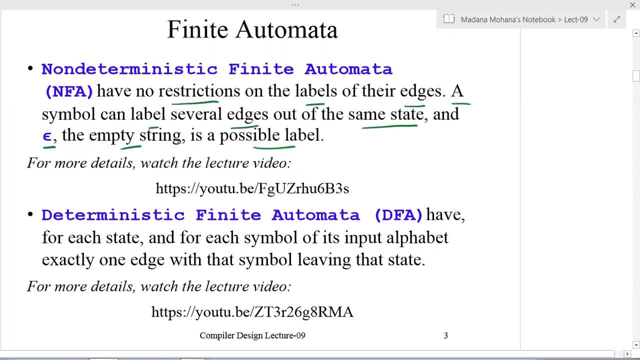 Similarly on deterministic finite automaton. we have restrictions For more details about the non-deterministic finite automaton you can use. you can watch the youtube lecture so which was covered in the previous semester in the course formal language and automata theory. Then coming to 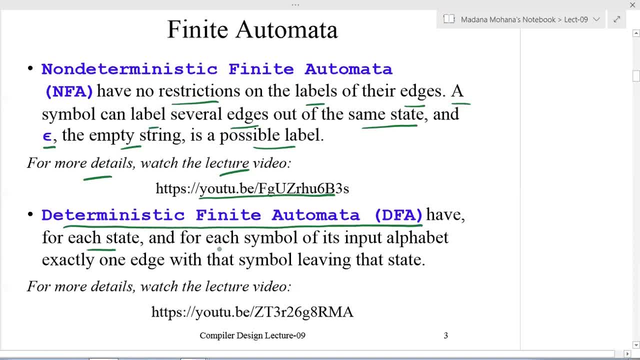 deterministic finite automaton how for each state and for each symbol of its input alphabet, exactly one edge with that symbol leaving that state. That means from a state on one input symbol it has only one next state, whereas in non-deterministic finite automaton, from a state on one input symbol it has more than one next state. with same input symbol, same state. 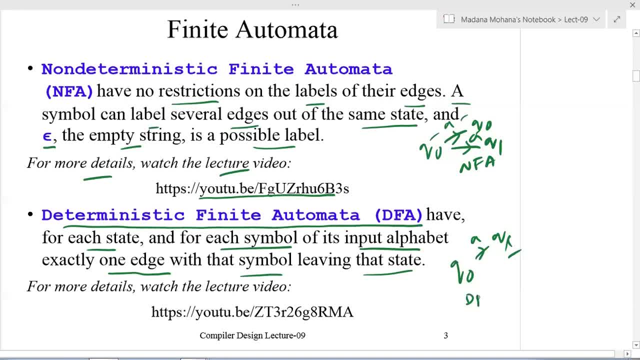 So this is called as NFA, This is called a deterministic finite automaton. Then, for more details about deterministic finite automaton, you have to watch the lecture video so which was covered in the previous semester. For more details about this, we have to watch the lecture video which was covered in the previous semester in the course formal language and automata theory. Then, coming to 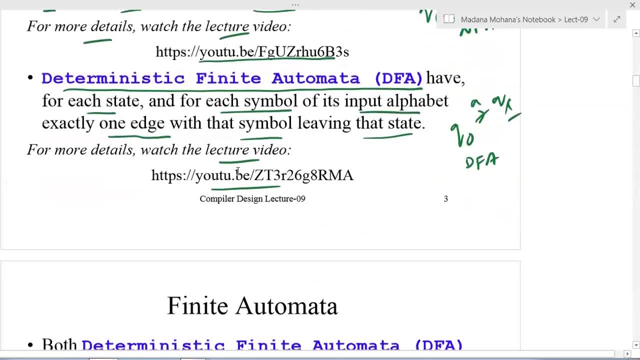 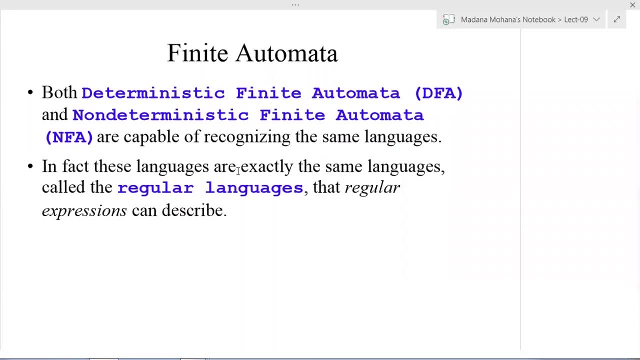 semester course: formal language and automata theory. so then, coming to some of the examples of this finite automata with acceptance. so both deterministic finite automaton and non-deterministic finite automaton which are capable of recognizing the same languages is one of the advantages of 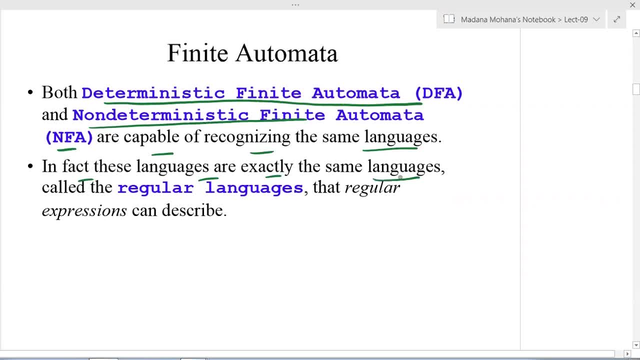 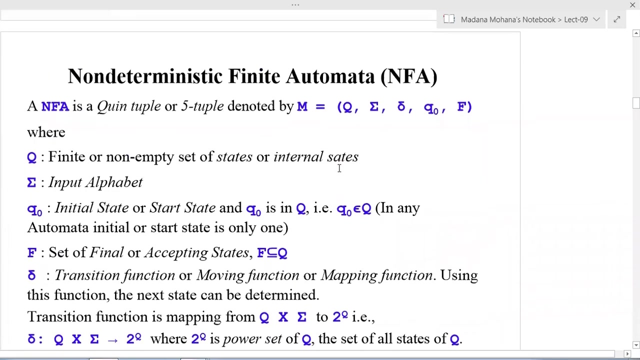 these two. in fact these languages are exactly the same languages called the regular languages that regular expression can describe. so both deterministic finite automata, non-deterministic finite automata accepts or recognizes regular languages, regular languages that regular expression can describe. then recall once the definition of these two automatons. first see the non-deterministic. 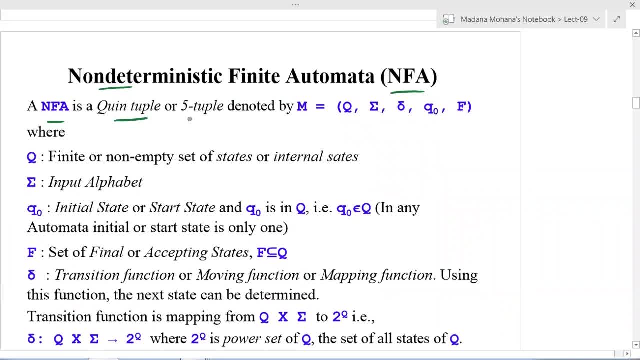 finite automata which can be defined as a quintuple or a fightable denoted by m equal to q, sigma, delta, q naught, f, where capital q is finite or non-empty set of states or internal state where a sigma is input alphabet, then q naught is initial state or start state and q naught is in. 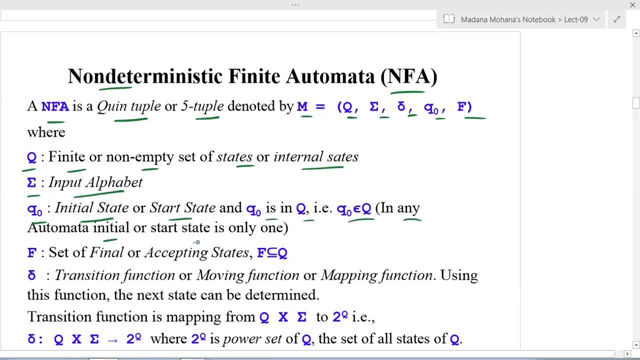 q, that is, q naught belongs to q. in any automaton, initial or start state is only one, then capital f is set of final or accepting state, which is subset of q. f is subset of q, then delta is transition function or moving function, also called as mapping function. using this function, 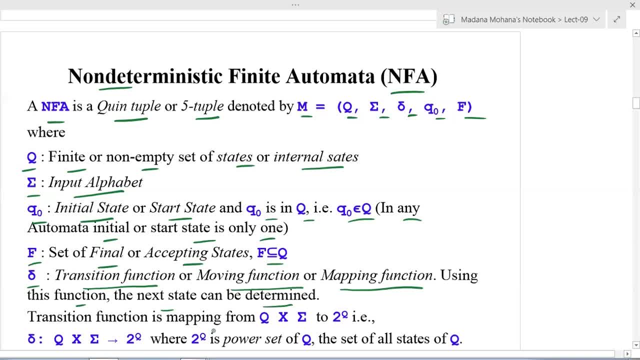 the next state can be determined, then the transition function is a mapping function which can be defined as mapping from q cross sigma to 2 power q, that is, delta, is mapping from q cross sigma to 2 power q, where 2 power q is power set of q, so which is the set of all states. 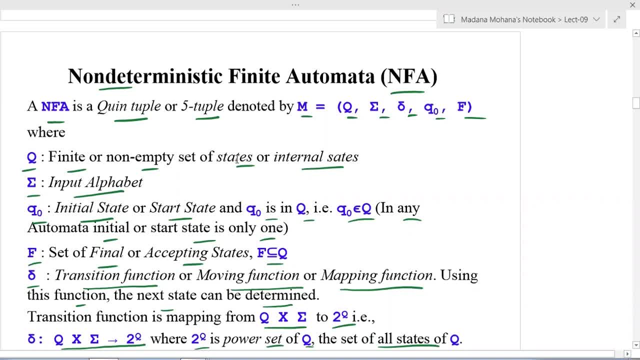 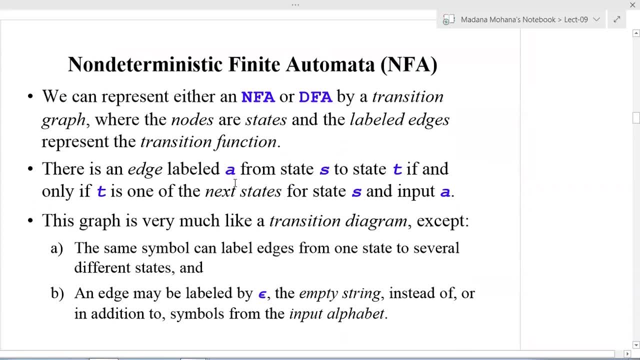 of q. this is the formal or mathematical or tuple definition of non-deterministic finite automaton. then deterministic finite automaton is also same, only the restrictions it has to follow. so we can represent either an nfa or dfa by a transition graph where the nodes are states: 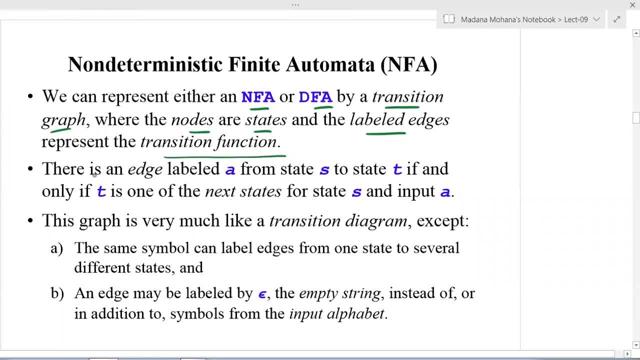 and the labeled edges represent the transition function. there is an edge labeled with a from state s to state t. if, and only if, t is one of the next states for the state s and input a of t is considered to be an infinite difference. this graph is very much like a transition. 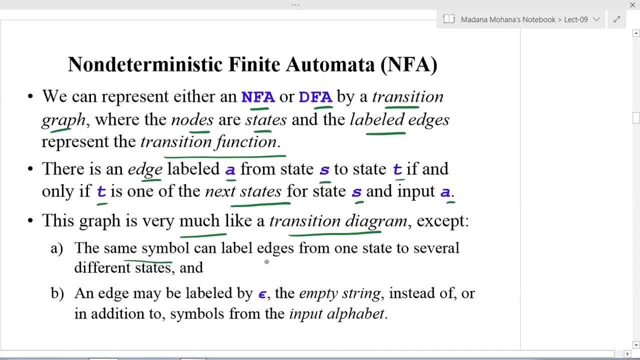 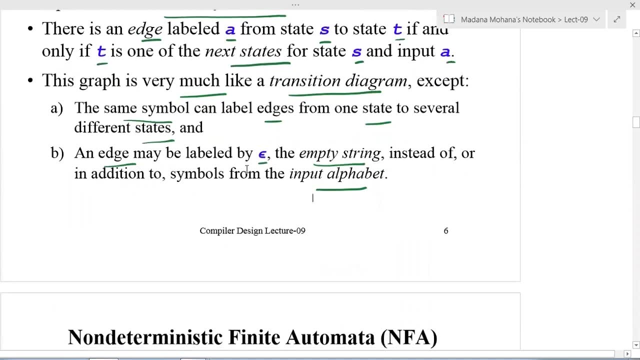 diagram, except the same symbol can label edges from one state to several different states, and an edge may be labeled by epsilon, which is the empty string instead of or in addition to symbols from the input alphabet. then let us see one example of non-deterministic finite. 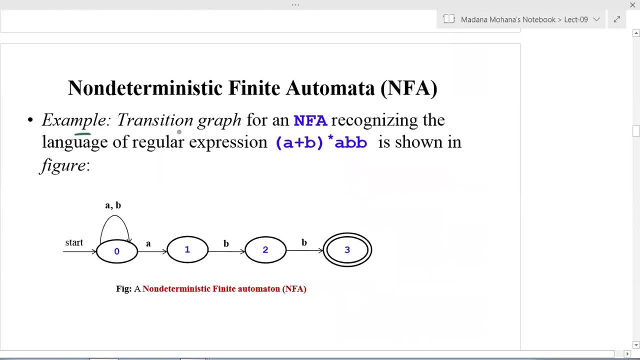 automaton transition diagram. so example transition graph for a non-deterministic finite automaton. transition diagram for a non-deterministic finite automaton is a transition diagram you non-deterministic finite automaton which recognizes the language of regular expression, a plus b, whole, closer a, b, b is shown figure. So the following automaton is for the regular: 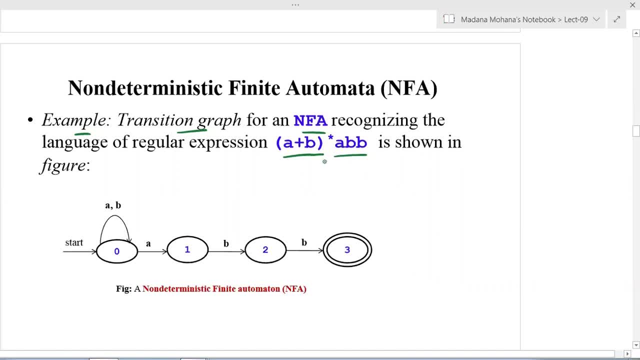 expression a plus b, whole closer. concatenation with a b, b. So now here we have, taken the first starting state, named as 0, labeled with the phrase start by drawing an arrow which denotes the starting state. So a plus b, whole closer can be written as a loop wherever plus is there, that is. 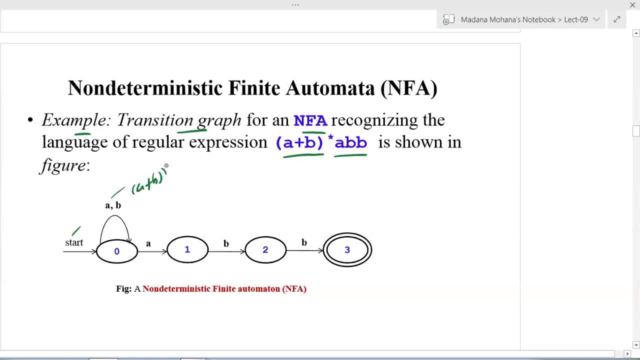 replaced with comma. This is nothing but a plus b, whole. closer Then here, by excluding epsilons directly. we are writing NFA here for simpler forms, Then for concatenation with a, b, b Concatenation means, you can take a sequence. So then now for this concatenation with first a. 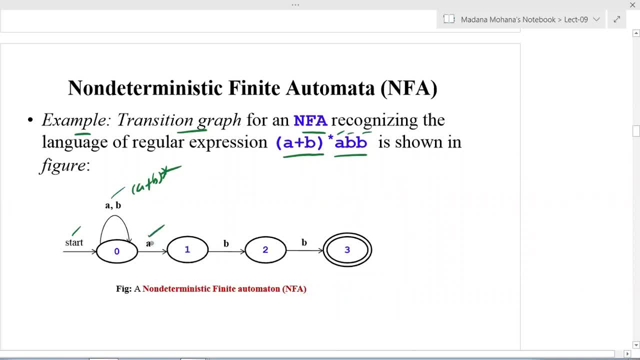 in between, by introducing a new state labeled with a, Then again introduce another state named 2.. Then the next label is the next symbol, that is b. Again introduce another new state, name it as 3.. Then the last symbol is b, Now the last state. 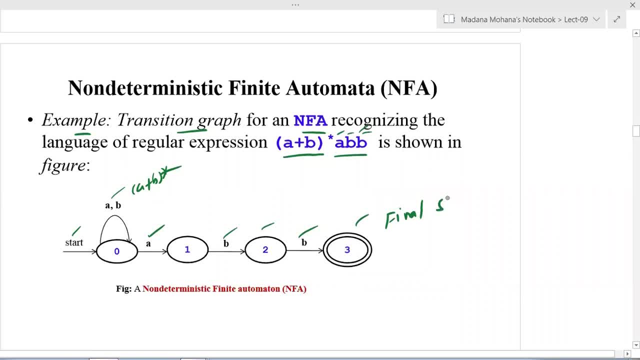 can be designated as final state which can be represented using double circle. Now you can see, whenever you can concatenate all these, what you will get here. this is loop means. here you will get a plus b whole closer. then concatenation with a, then again concatenation with b, again concatenation with b. now you see here. 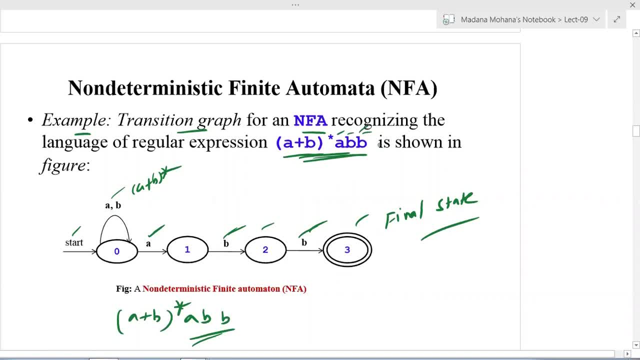 we got our regular expression. what are the given regular expression? So this is the example of non-deterministic finite automata. you can test why- why not? is a deterministic finite automata? How can you say it is non-deterministic here? Let us see from state 0. see on input a. 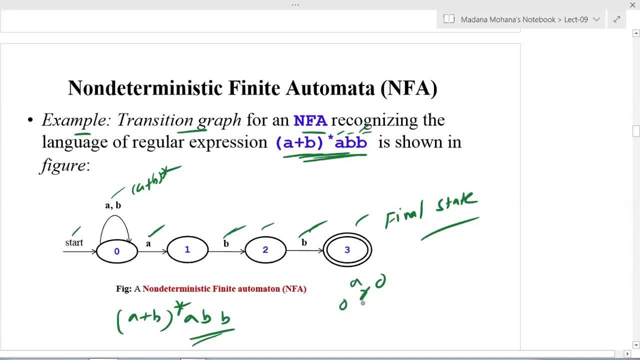 it is going to state 0. same again on input a: it is going to state 1.. So that is why this is here. That is the format theаго that will be. I mean this: b is going to start 0 again and input into state 1.. 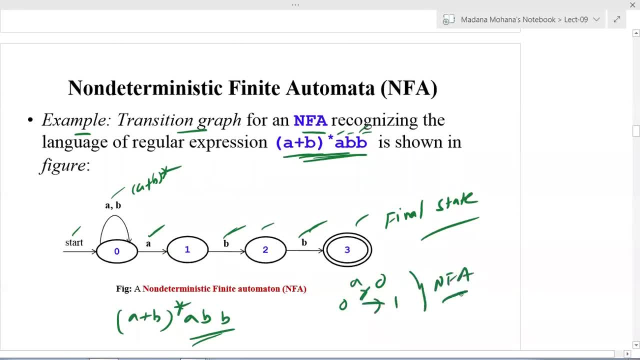 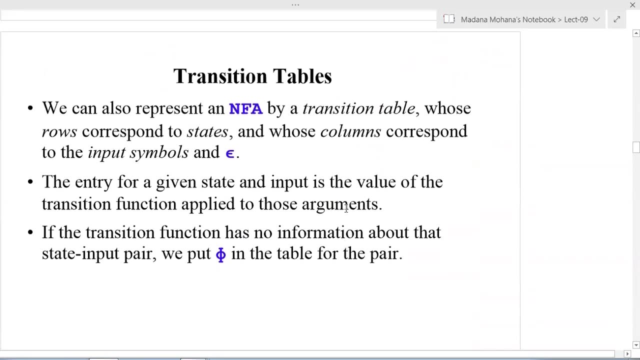 one. so that's why this is nfa in deterministic finite automata. this is not allowed from your state with same input symbol. it has only one next state even it doesn't allows null. also, that's why this is example of non-deterministic finite automata. then, similarly, we can construct a: 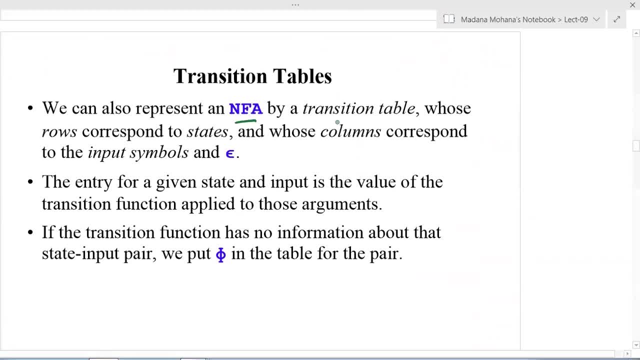 transition table. also, we can also represent an nfa by a transition table whose rows correspond to states and whose columns correspond to input symbols, including null. then the entry for a given state and input is the value of the transition function applied to those arguments. if the transition function has no information about that state input path. state input path delta. 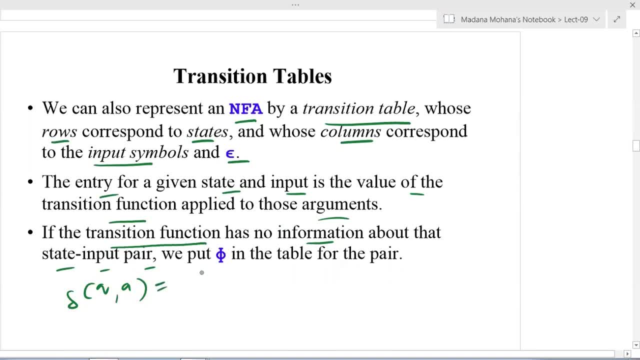 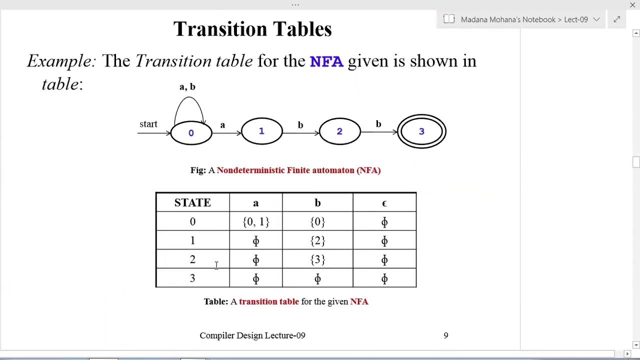 so no information, that means no transition. then simply we can put pi in the table first, this way on state q, on input a. so some cases we will use simply blank or iphone, but generally we will put pi also. now let us see for the previous example the transition table. 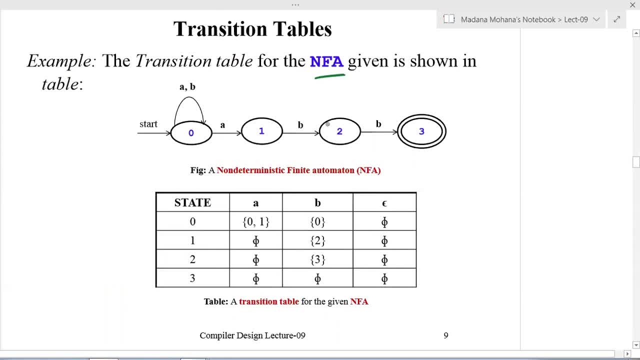 the transition table for the nfa given below. so same nfa is constant. now the transition table. here we will take rows and column combinations. so here the row heading are states, then column headings are the input symbols which can be taken from sigma. then including null also, but null is not in sigma, there is not input alphabet, so that is separate. 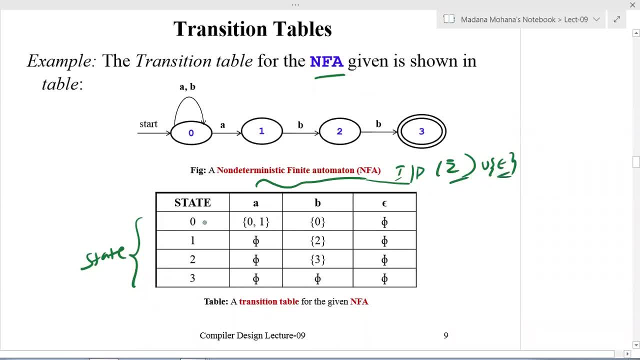 empty string. so for this also you can define transition from state q- naught. see on input a: it is going to q naught and it is going to i mean 0 and it is going to 1.. so now we can combine states 0 comma 1.. here don't confuse: 0, 1 to 3 are state names, whereas abr input symbols. 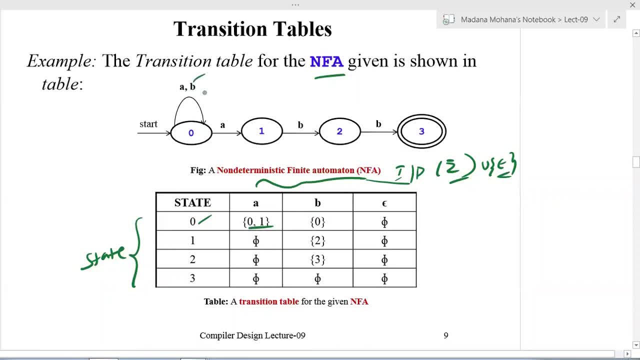 then from state 0 on input b, it is going to 0 itself, therefore 0. then from state 0 with epsilon, you don't have any transition labeled with epsilon, that's why we have made it as 5. then from state 1 on input a, you don't have transition, so it is 5.. then on input b, it is going to state 2. 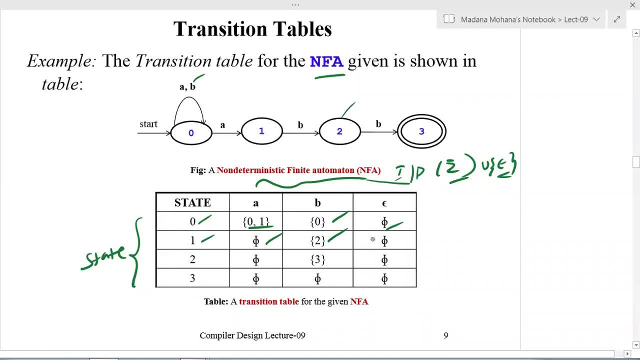 therefore the next state is 2.. then from state 1 with the epsilon you don't have transition. why you have taken epsilon means because this is nfa, there is possibility to have epsilon also. that's why we have taken epsilon, whereas dfa. you can't consider epsilon as the column heading in the 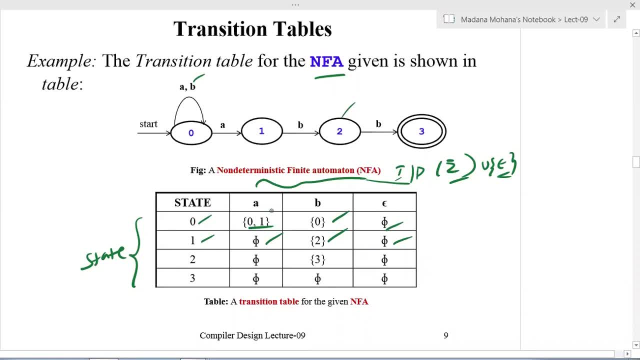 transition table. then from state 2 on input a, you don't have transition, so it is 5.. from state 2 on input b, it is going to state 3, therefore it is 3.. then from state 2 on epsilon, you don't have transition. from state 3 on input a b, you don't have transition, so both are pi. 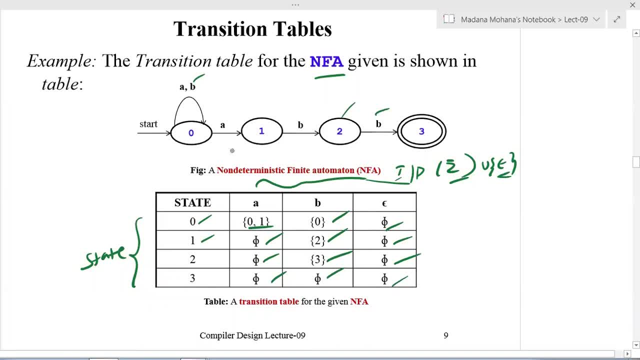 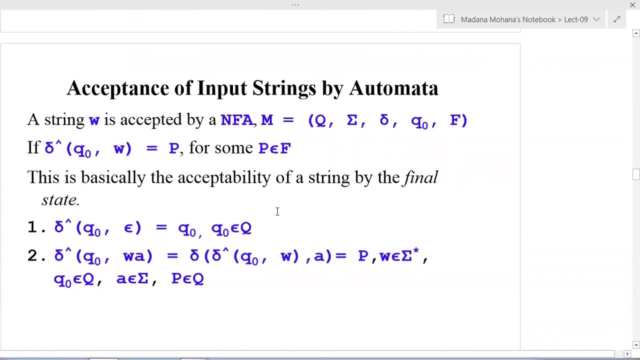 then on epsilon also, there is no transition. so this is 5.. now this is the transition table for the given nfa. so now let us see acceptance of input string by automata: same concept, whatever we discussed in the course, formal language and automata theory. same concept term we are using here. 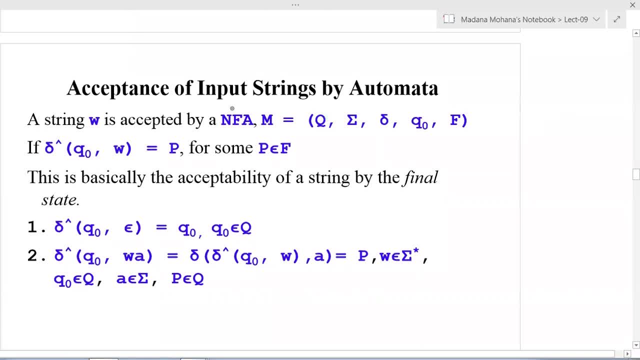 so acceptance of input string by final uh finite automata. it may be nfa or dfa, whatever a string w is said to be accepted by a nfa m equal to q sigma delta q naught f. the condition is if delta cap of q naught comma w equal to p, where delta cap is the extended delta definition of nfa. so whenever 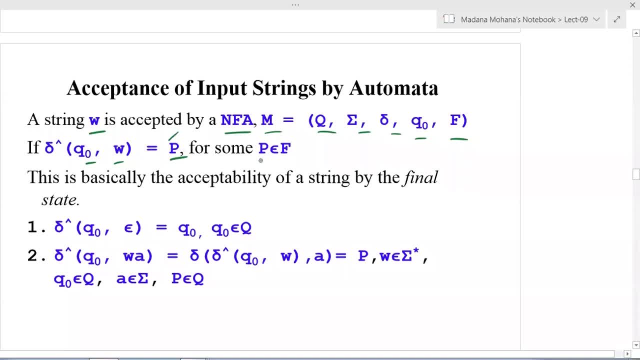 you will get a state p or set of states. therefore some p belongs to f from the set p, at least the set p belongs to f from the set p, at least from the set p belongs to f from the set p. at least the one state is in a final state. then you can say: the string w is accepted by this nfa. so this: 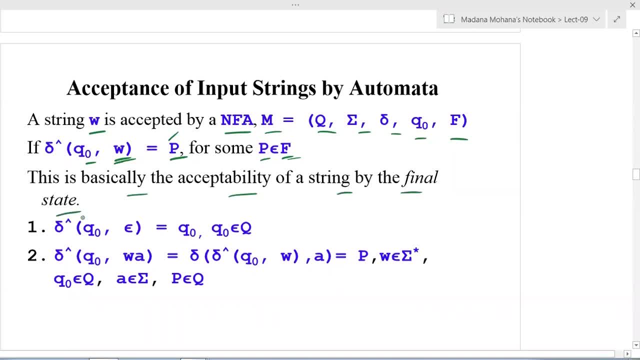 is basically the acceptability of a string by the final state. so as for the extended delta definition, these two rules are used while checking the acceptance of input string by automata. the first condition is delta, cap of q, naught comma, epsilon. so from a state- initial state- with the 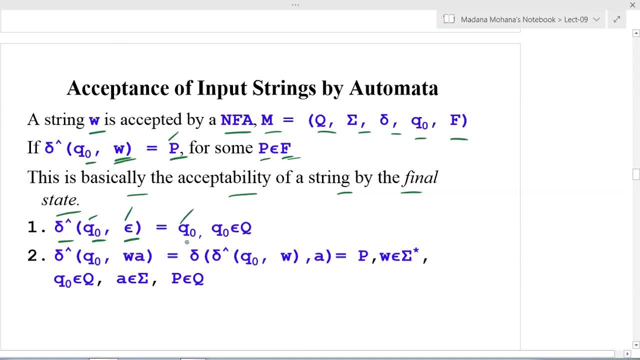 empty input. so here there is no change of state. simply you will get same state. so you will get q naught only where q naught belongs to the set capital, q set of states. then second rule: delta cap of q naught, comma testing w, followed by an input symbol a. this can be expanded like this: 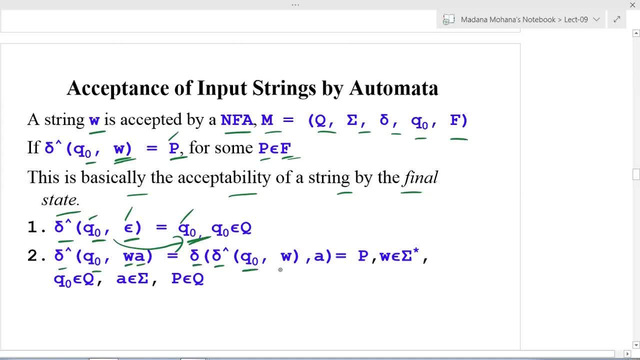 by using normal delta delta of delta cap of q, naught, comma w, comma a. here w and a are separated after simplification of this by repeating this rule. finally, if you will get a set of states denoted as capital p, so where w belongs to sequence. 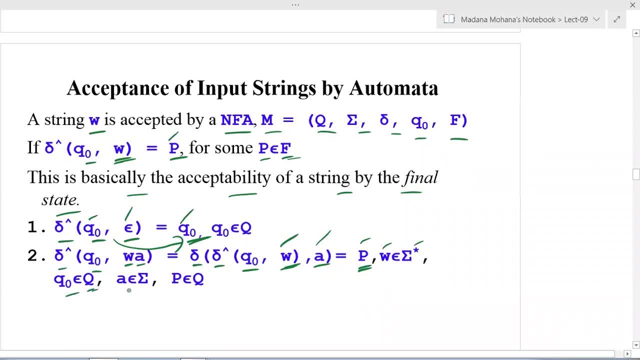 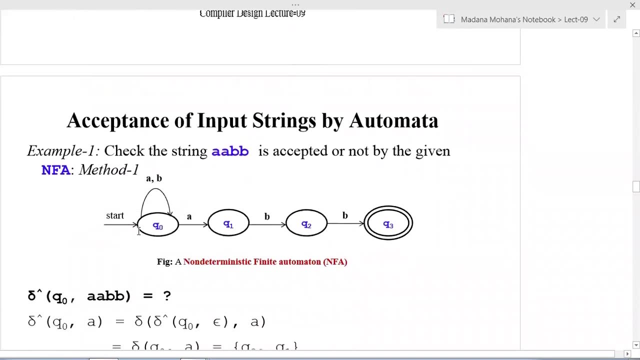 sigma closer the string, then q naught belongs to capital q, then a belongs to sigma input alphabet, then p belongs to q. so by using this rule, one and two during acceptance of strings by automata. so we will verify. now let us check the same example, what we described above: check the string. 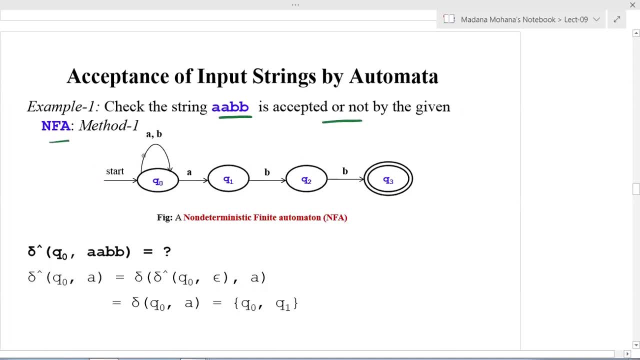 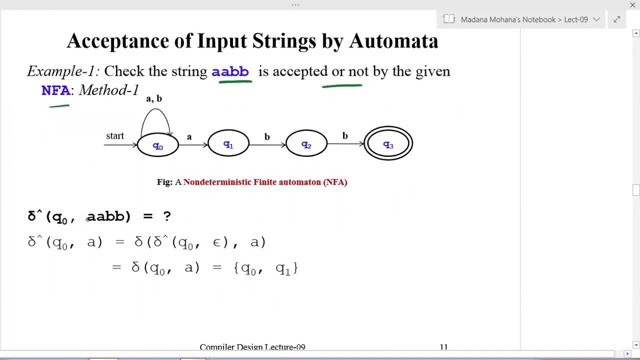 a, a, b, b is accepted or not by the given nfa. so the method one. here what you have to do is simply by taking the given input string with extended delta, definition, delta, cap of q, naught, comma a, b. so here, first, what you have to do, the left over input symbol we will take. 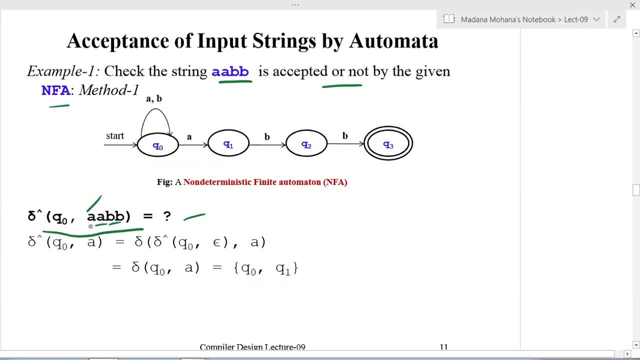 then two symbols we will take, then three symbols we will take, then four symbols like that. first input symbol, a leftmost symbol you can take. you can apply this external delta definition, so delta capital q, naught comma a, using the above extended delta rules. this can be expanded by using: 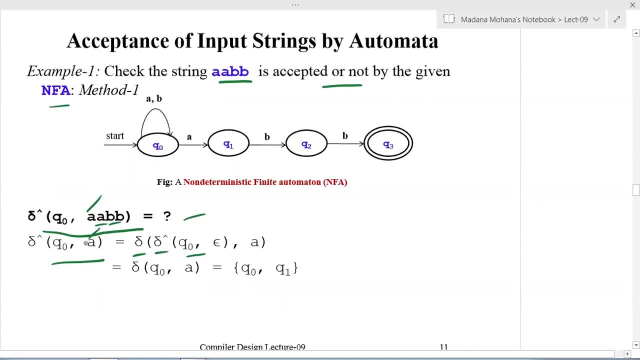 delta, delta, delta, capital separating a. whenever a is separated, then what will be there here? null epsilon, comma a. you know this value. so delta cap of q naught comma epsilon equal to q naught, using the above rule one. so you can substitute this value as q naught. so this entire value is q naught comma. now the input is: 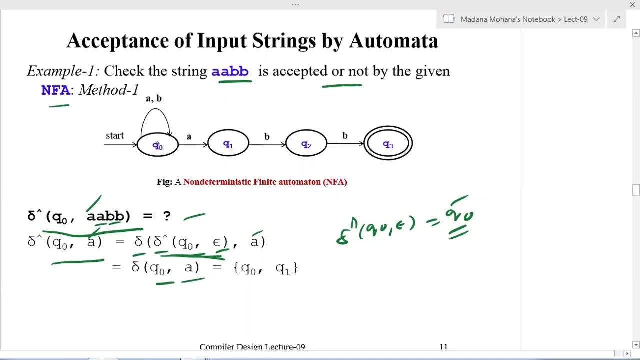 a. now delta of q naught on a by the given nfa. what is the delta of q naught on a? it is going to q naught and it is going to q1. therefore, q naught q1. this is the result of the first step. 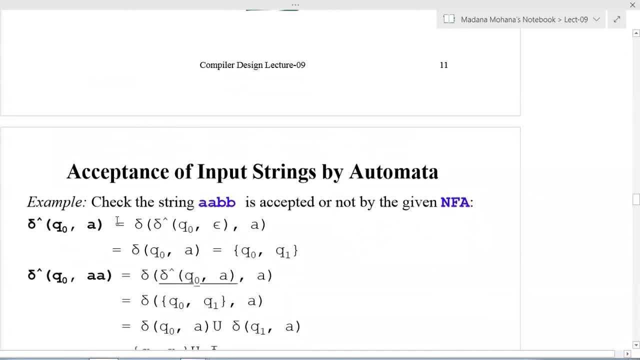 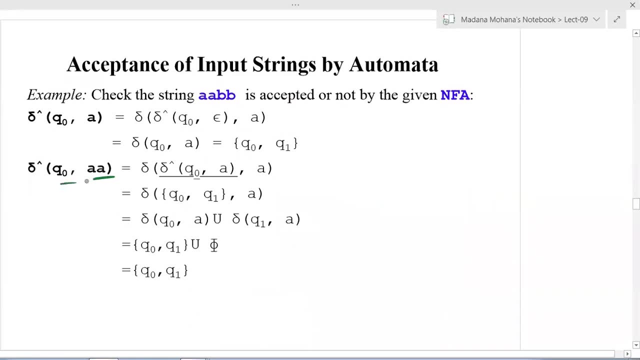 next step. you can take the two input symbols from left to right. so now second step. so here we will take two input symbols: delta, cap of q, naught, comma a. so again you can expand this one by separating the rightmost a. this can be written as a delta of delta, cap of q, naught, comma a comma. 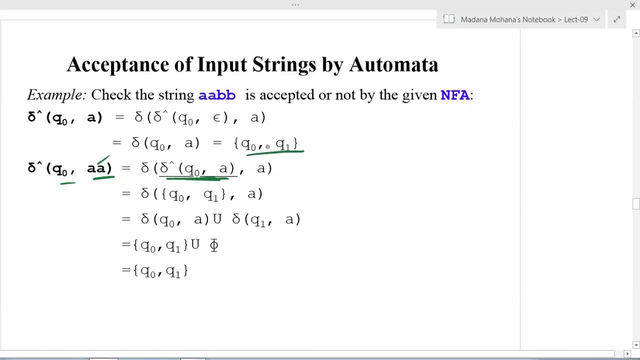 a. we know this value in the previous step. what is this value? q, naught, q1. substitute this value and we can take the two input symbols from left to right. so now, second step. so here value. now this will equal to delta of q, naught comma, q1 comma. input is a. again, apply union rule. 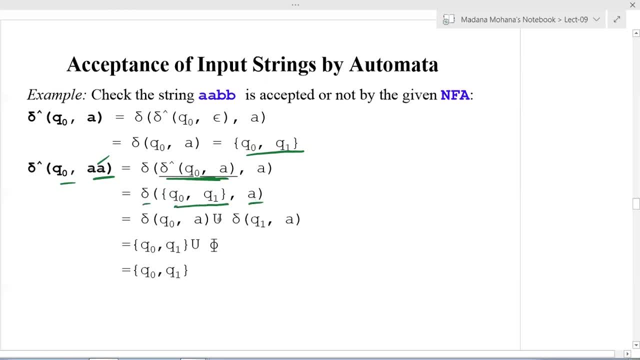 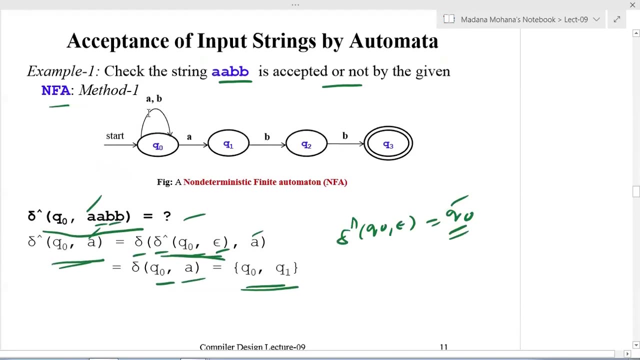 here this can be written as delta of q naught comma a, union delta of q1 comma a. so then substitute these transitions by using, by seeing the transition diagram or table. so here the first one is q naught on a q naught on a equal to q naught comma q1, q naught comma q1, then q naught. 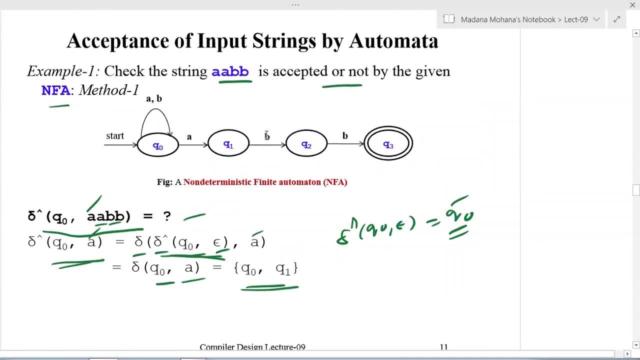 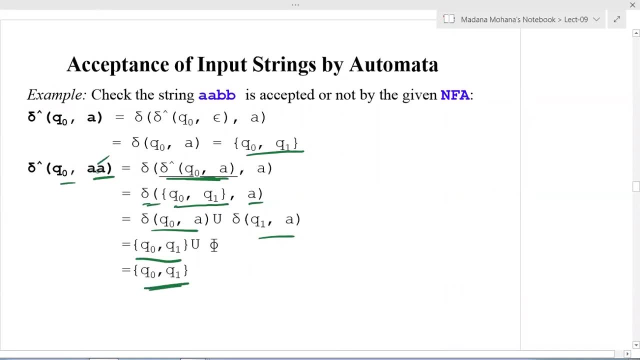 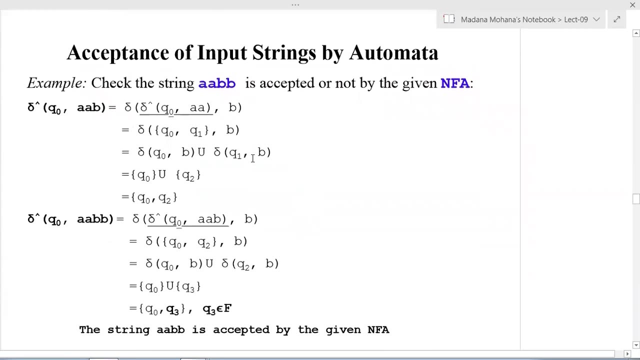 on b as well, q1 on a, q1 on input a. you don't have transition, simply you can take pi. now, by simplifying this one, you will get q, naught q1 only. so this is the second step. value, third step: then you can take three input symbols. the third symbol is b, is added. here again you can expand. 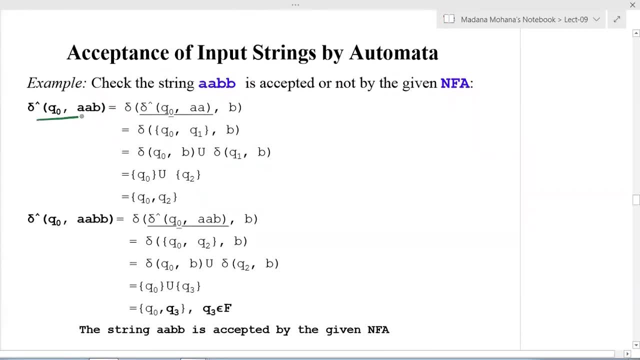 this one like that. you have to continue now. delta. cap of q, naught comma, rightmost symbol. every time we have to separate, so then this can be written as delta of delta. cap of q, naught, comma a, comma b. you know this value in the previous step: delta. 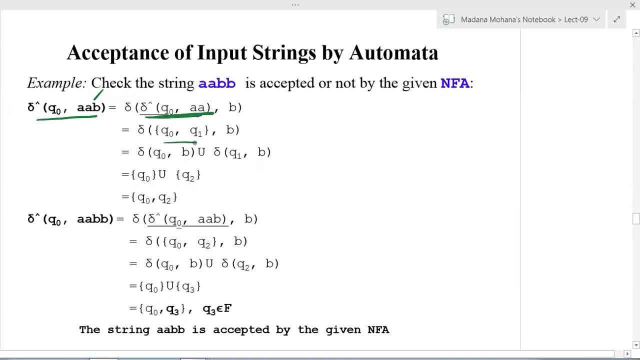 cap of q naught comma a. equal to q naught comma q1. this value is substituted. the next input symbol is b. again, you can apply union rule with the delta delta for q naught comma b. union delta for q1 comma b. now q naught on b from the transition diagram. its value is q naught, then delta of q1. 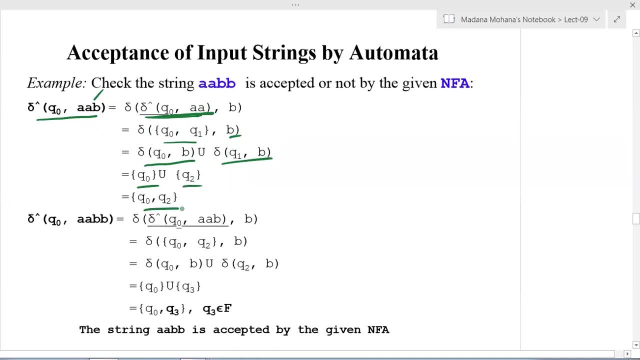 on b, its transition is q2. then by combining these two you will get q, naught comma, q2. then you can take the entire thing. why? because of a latter, only one symbol is missed. there is one more b now delta cap of q. naught comma a, a, b, b. now last b, rightmost b. 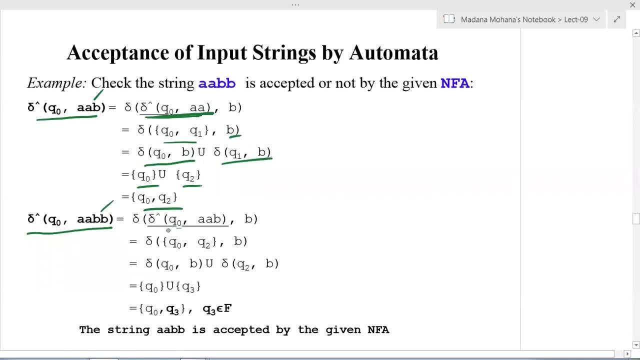 you can separate. now this can be written as delta of delta cap of q naught, comma a, a, b, b. you know this value in the previous step. what is this value? q naught comma q2. the input is b. now you can substitute here delta of q naught comma q2, comma b and, by applying union rule, delta of q naught on b. 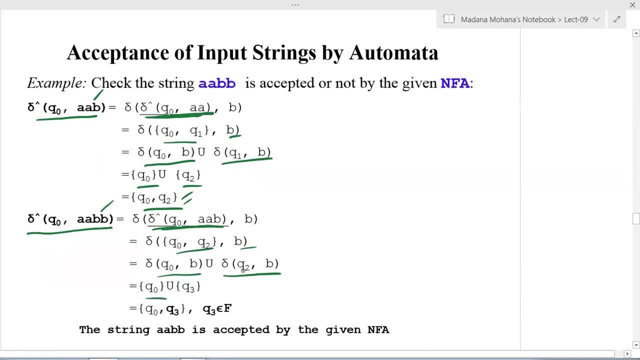 this transition: delta of q naught on b, you will get q naught. then delta of q2 on b, you will get q3. then, by combining this, q naught, q3. now you can see, let us assume this as capital p. this is the last. 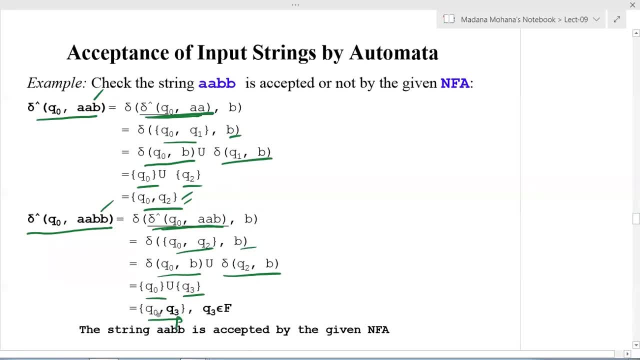 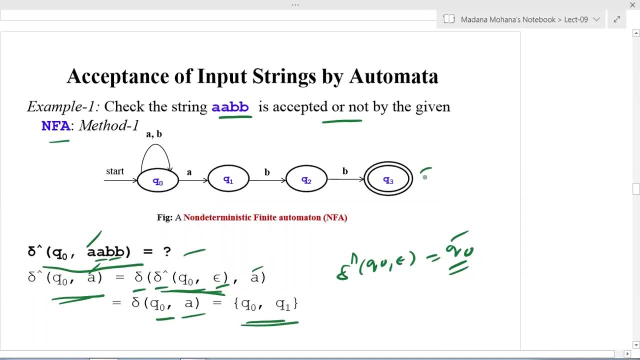 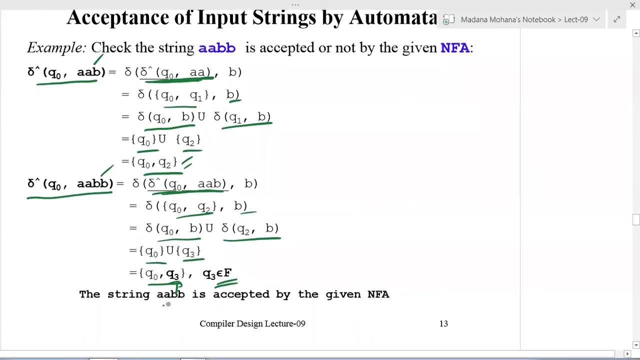 step. so in this at least some p belongs to f. here you can see we got q3. q3 is the final state. you can see the transition diagram here. q3 is the final state. therefore, finally, we got a state in. therefore the conclusion, the string a, a, b, b. 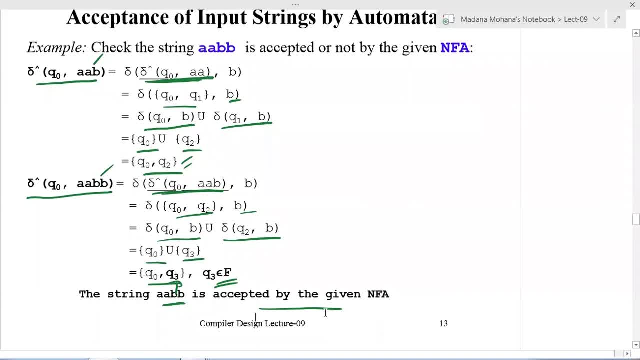 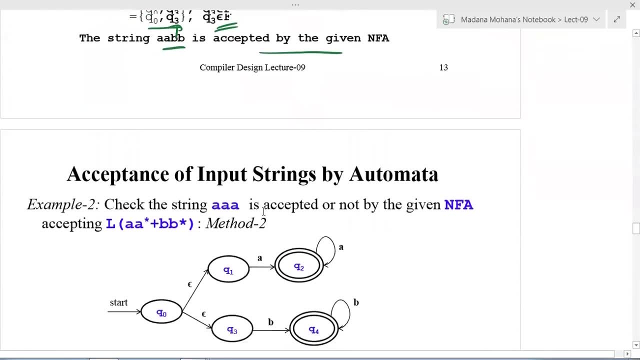 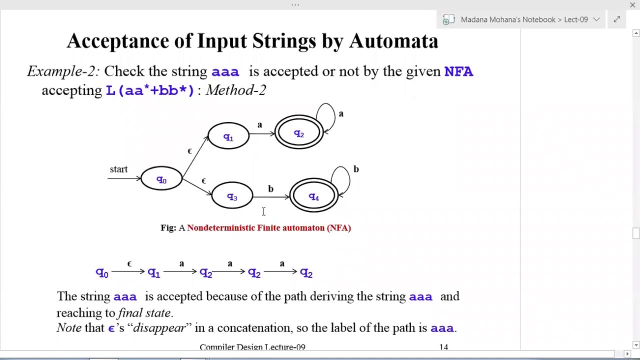 is accepted by the given non-deterministic, finite automata. like that we can check any given string, whether this is accepted or not by the given automata. so now we have another method also. so another method, nothing, but by using proliferation, a sequence of moves made. 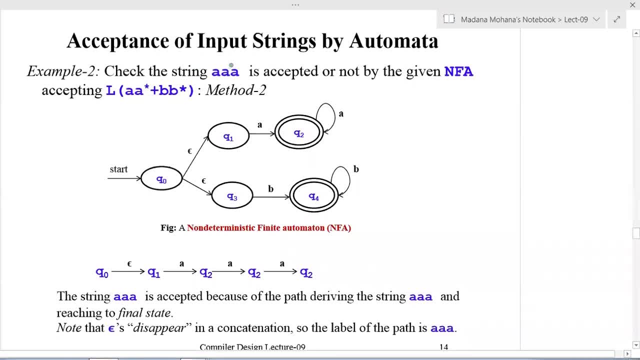 for the string to accept. so check the string a. a is accepted not by the given nfa, excepting long ways. this is the long ways: a a closer plus b b closer. this is another example actually, so here we will see the method two. we need to check triple a whether this is accepted. 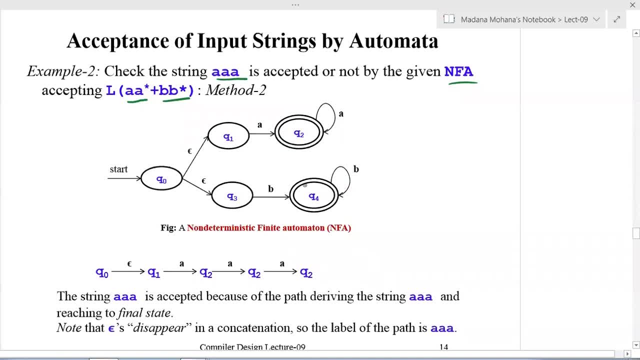 or not. same example. you can do it as practice problem using method one also. so here, first you can start with the initial state q naught. so first symbol, we need to derive a. the possibilities are in which path, if you will consider if you will get a. so from q naught to q1 with epsilon. finally, epsilon is avoided. why? because 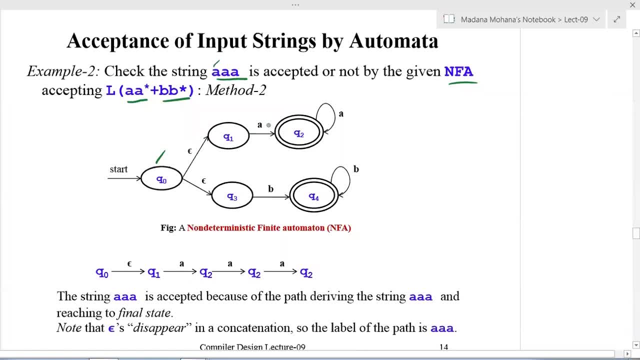 this is null. whenever you can go to q1, state here we will get a. then if you can go to q3, you won't get a. compulsory the possibilities. you have to go through q1 only. that's why q naught to q1, the first. 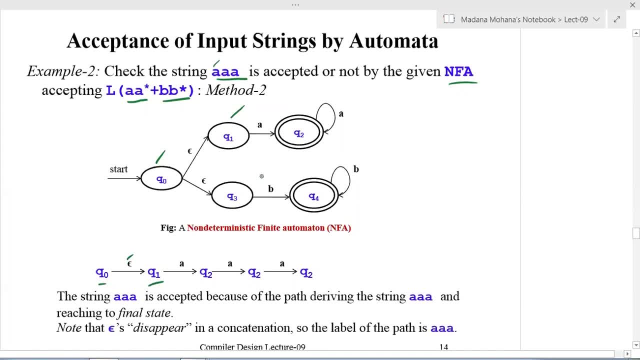 path labeled by epsilon. then from q1- compulsory- our input is a. so anyway the transition is also a. so from q1 to q2 it is going to q2. so then from q2. again it contains a as loop. so if you want any number of a's you can take. so now you want one more a from q2 to q2, take a. then again we need: 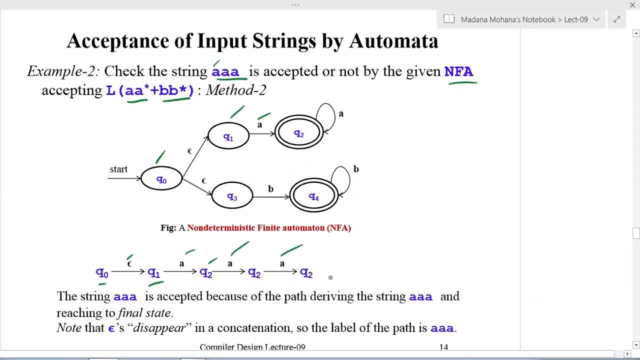 one more: a, q2 to q2, a. now you can combine in the sequence the input symbols. what are the symbols by excluding null? a, a, a. now you can see. so we derived the string. but in this sequence the last one, q2. that should be a final state here. q2 belongs to f, also here. 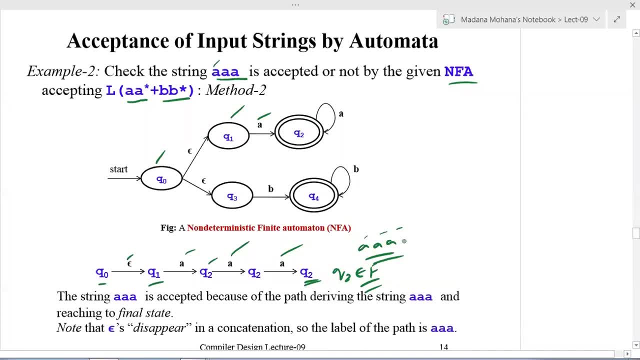 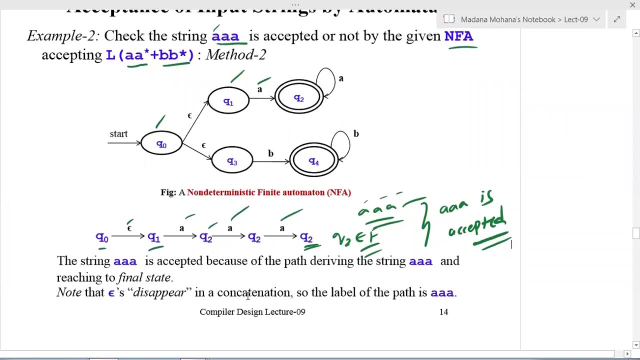 q2 is final state, which is represented with the double circle. therefore we derived the string, then we got the final state. therefore the string a- a is accepted. like that by writing the sequence of paths also we can check accepted. the string a- a is accepted because of the path deriving the. 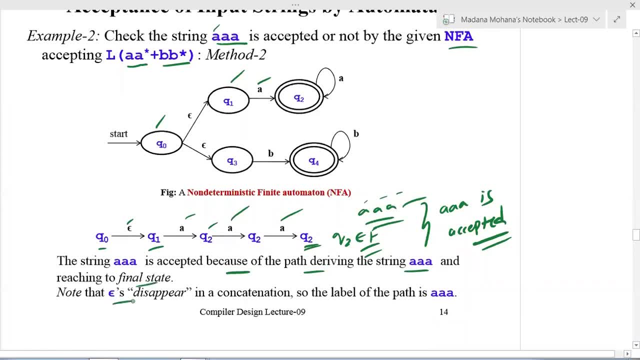 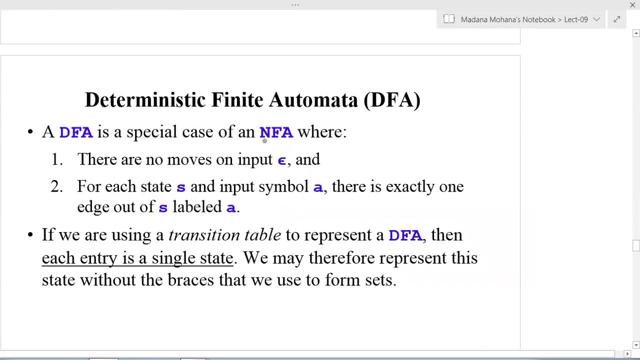 string a and reaching to the final state, note that epsilon disappear in a concatenation. so the level of the path is triple a. this is the method q- previous problem also you can do using this method, then coming to deterministic finite automaton. so this is the special case of nfa. 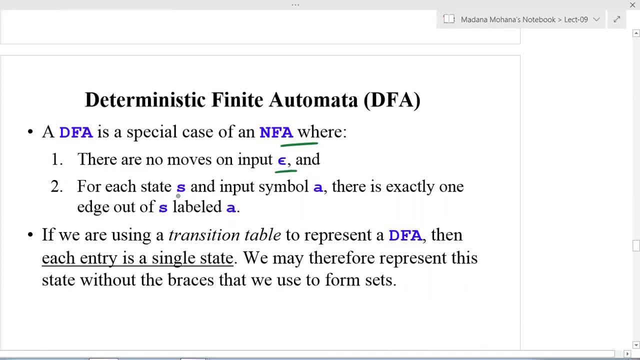 where there are no moves on input epsilon and for each state yes and an input symbol a, there exists exactly one edge out of s labeled a. so if you are using a transition table to represent a dfa, then each entry is a single state. we may therefore represent this state without a braces. why? because 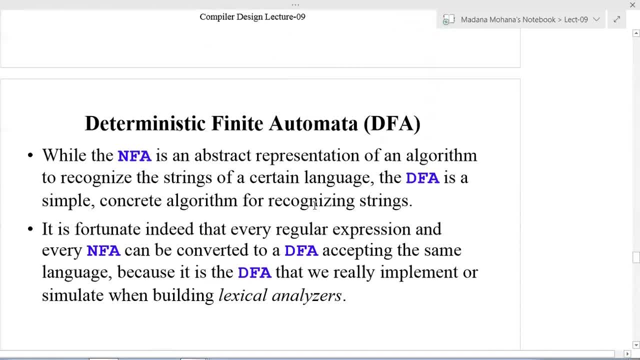 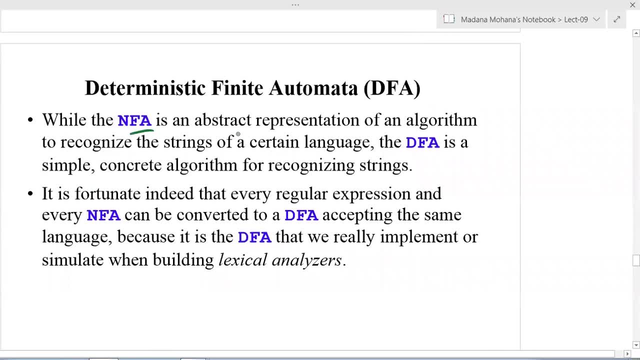 only one next state that we use to form sets. so now, deterministic, finite automaton. this is some differences between nf and dfe. while the nf is an abstract representation of an algorithm to recognize the strings of a certain languages, then the dfe is simple, concrete algorithm for recognizing strings. so it is fortunate indeed that every regular expression and every 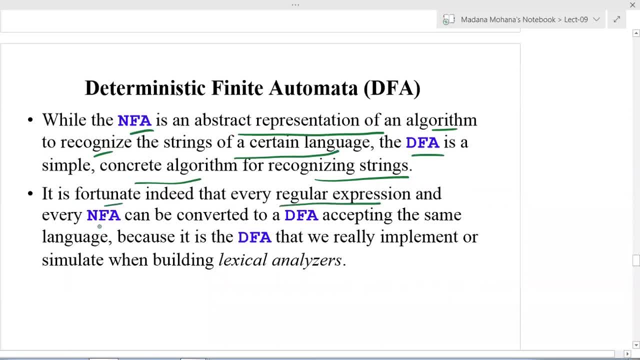 and your dum before Brittany is great for class and then, on the other hand, you will not get any forj jorle of ketumettai. since that you knowuesta. data Check out headquarters table won't allow data Check out headquarters. data Check out headquarters data. Check out headquarters. видно sri hair without. 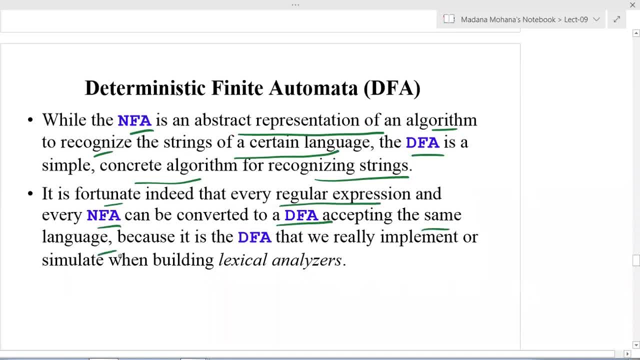 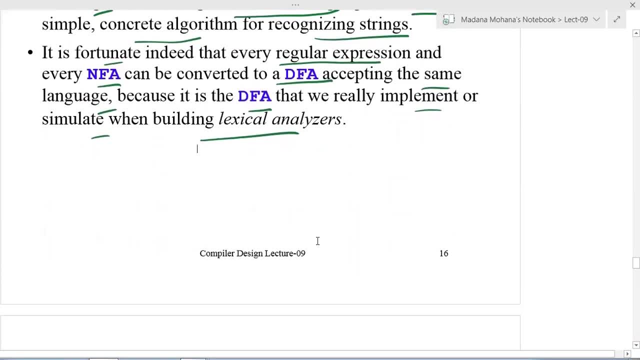 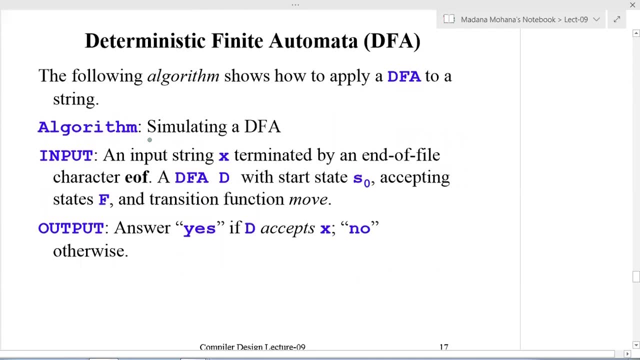 NFA can be converted to a DFA accepting the same language, because it is the DFA that we really implement or simulate when building a lexical analyzer. So then here a simple algorithm for simulating a DFA is shown here. the algorithm name is called as simulating a deterministic finite automaton. the input is an input string x, terminated. 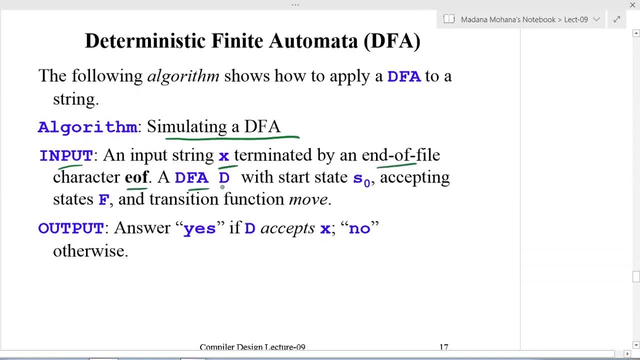 by end of file using the character EOF, then a DFA named as D, with the start state: assume S, naught accepting state, assume capital F and transition function: assume it has moved. then output is the answer yes if D accepts x, otherwise no. So output of any automaton is S or no, accept or not accept. then the method is: apply the 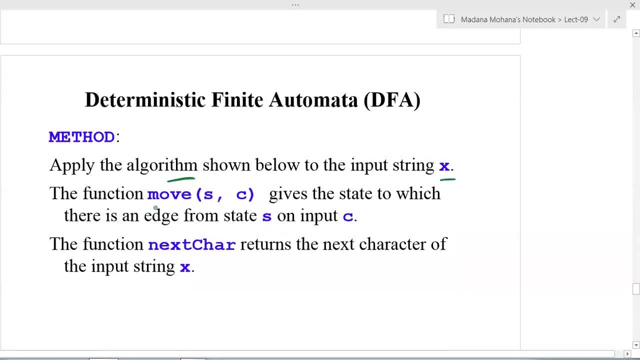 algorithm shown below. to the input string x, the function move of S comma C use the state to which there is an edge from state S. on input C, The function next character Returns the next character of the input string x. so here move and next character, two functions. 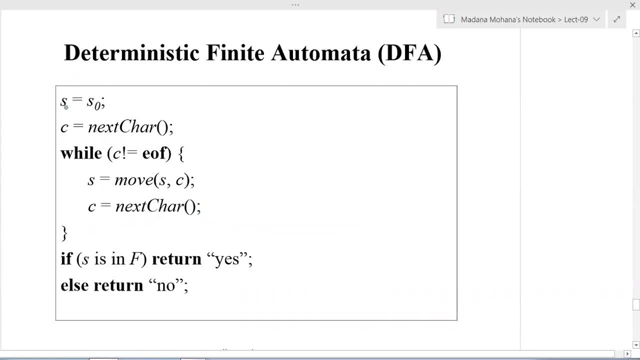 are used. now let us see the skeletal algorithm: first S equal to S naught, then C equal to next character. this is the method we are calling: while C naught equal to end of file, then S equal to move S comma C, then C equal to next character, then if S is in final state, then 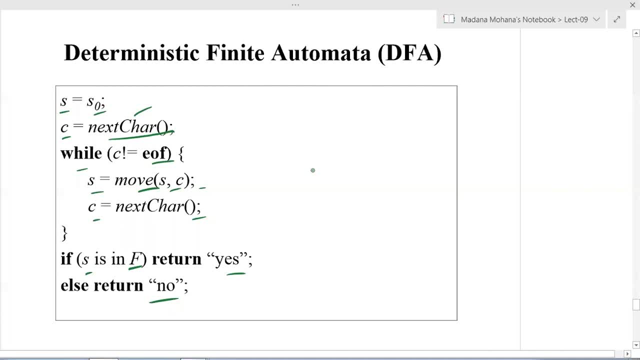 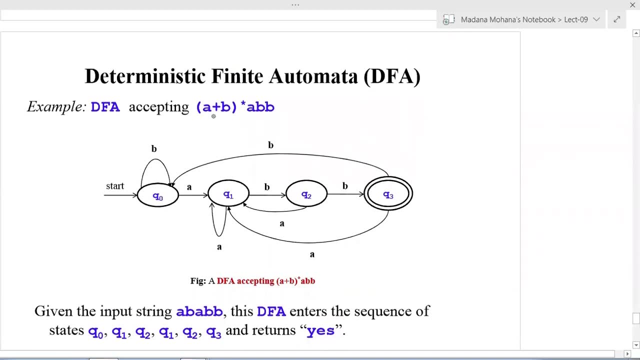 it returns S, otherwise it returns no else. no, this is the simple. So the next one is the formula for DFA. So then let us see one example of DFA accepting the long ways the regular expression A plus B, whole closer A, B, B. in the previous example for the same regular expression we discussed, 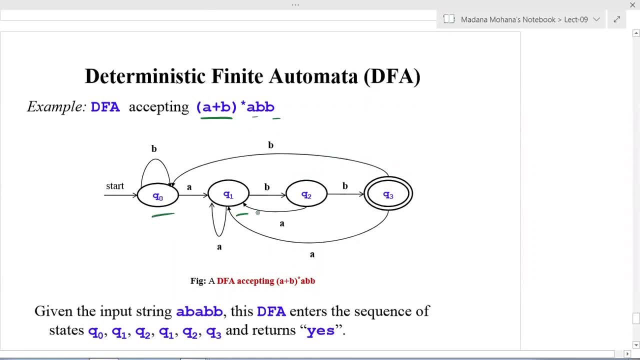 the NFA, for that the equivalent DFA is constructed. so how to construct this DFA for the given NFA? we know the procedures: NFA to DFA conversions. even if we have epsilon NFA with epsilon two DFA also, using those methods you can construct the DFA again. we will use the subset method. 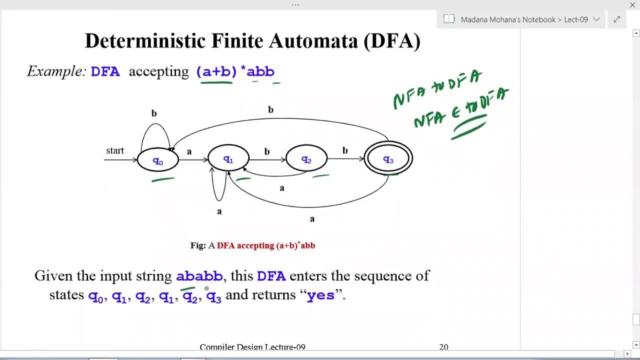 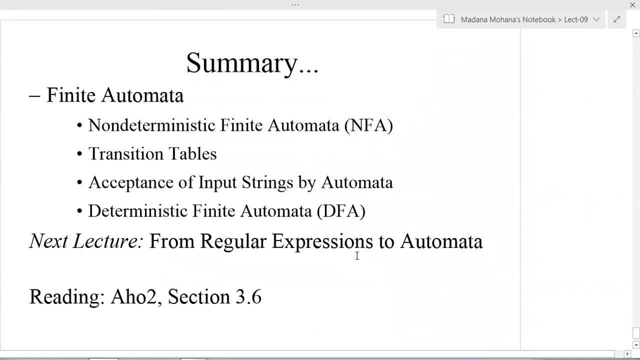 also that we will discuss later Now here, the given input string A, B, A B B. this DFA enters the sequence of states to get this string Q naught: Q 1, Q 2, Q 1, Q 2, Q 3, and finally it returns S. now coming to the summary of. 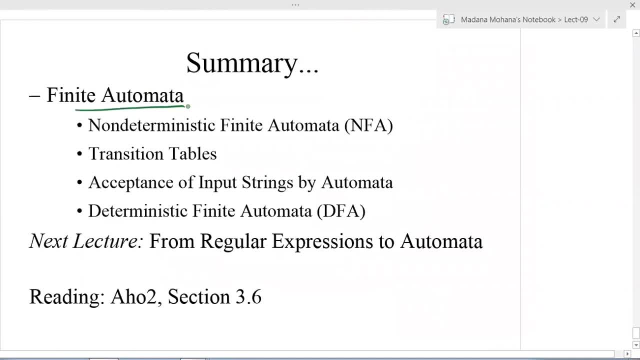 this lecture. here we discussed about first introduction to finite automata, then we discussed about non detrins finite automaton, then transition table, then an example, then acceptance of input string by this automaton, then deterministic finite automaton. So next lecture we will discuss about from regular 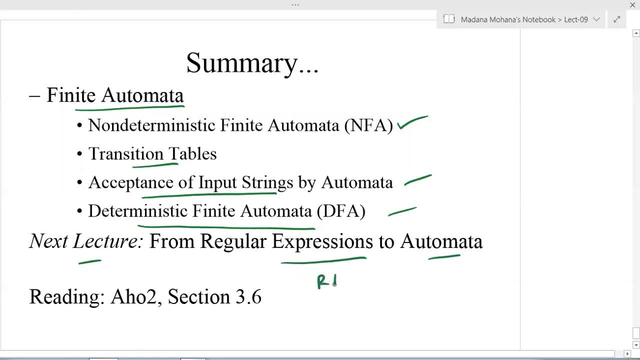 expression to automaton. Suppose, if we have a regular expression, conversion of regular expression to first we have a NFA or NFA with epsilon, then direct DFA. So these three conversions we will discuss in the next lecture. This also we covered in our previous course. formal language. 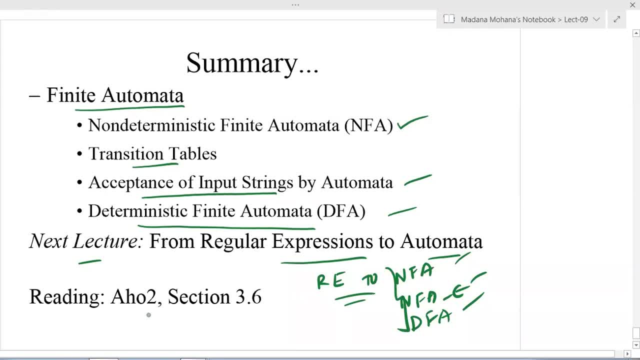 and automaton theory. So for this lecture, the reference Aho to section 3.6. whatever we covered in this lecture, Now I stop here. we will meet you in the next class with the new topic.